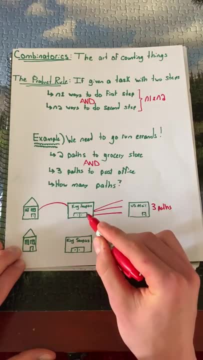 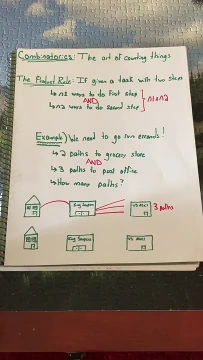 way to the post office, or this one way to the post, the grocery store and this final way to the post office, In total three paths. Now let's suppose we take that other path to the grocery store. Again, there are three paths we could take to the post office. 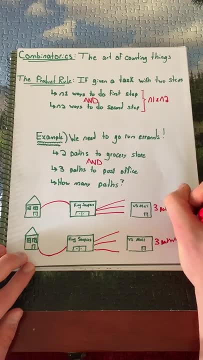 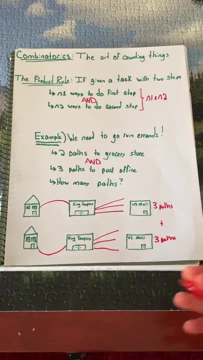 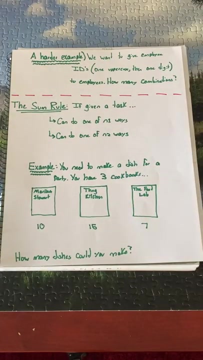 and there are three more paths. That gives us three plus three paths, or six paths that we could take. So there, we've validated the product rule. Now you'll probably get some harder problems than that, so I've decided to go over a harder example as well. Suppose we wanted to give out employee. 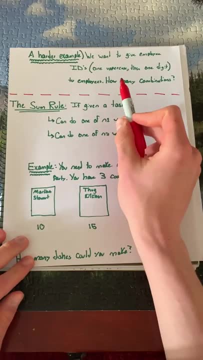 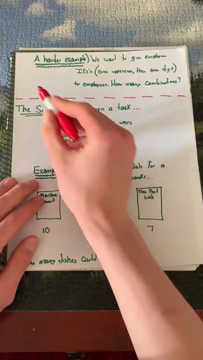 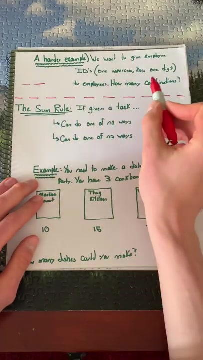 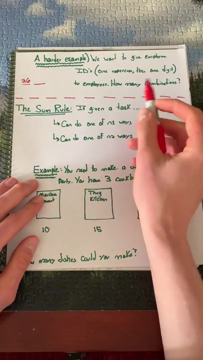 ids to employees. An employee id consists of one uppercase letter followed by one digit. How many combinations or how many ids can we make? We know that id consists of two characters. This first character needs to be an uppercase letter, of which there are 26.. The second character needs to be a digit, and there are 10 digits. 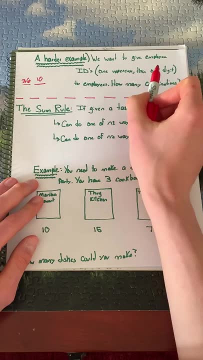 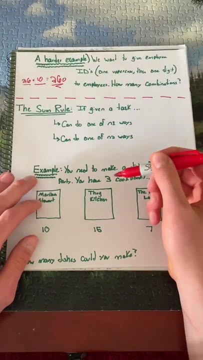 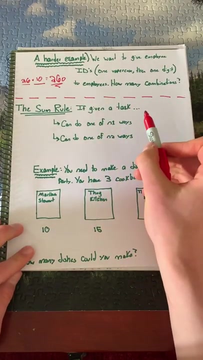 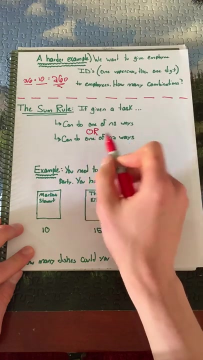 Using the product rule, we know we need one uppercase and one digit. so we get 26 times 10 equals 260 total ids. Now let's go over the sum rule. The sum rule states that if we're given a task and we can do the task one of n1 ways, or we can do the task one of n2 ways. 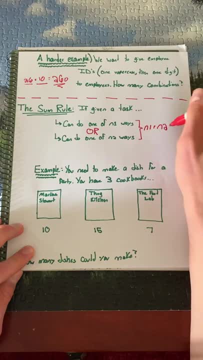 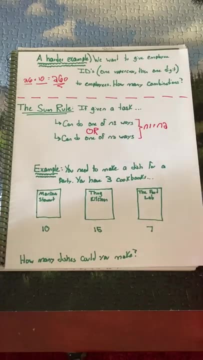 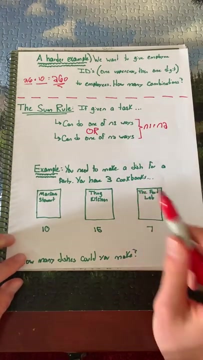 then there are n1 plus n2 ways to do the task. Again, notice I point out the keyword. or here, When you see that keyword, you're going to want to be thinking sum rule. So again, let's do an example problem: You need to make a dish for a party and you have three cookbooks. 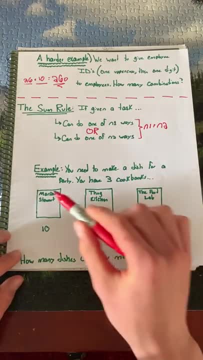 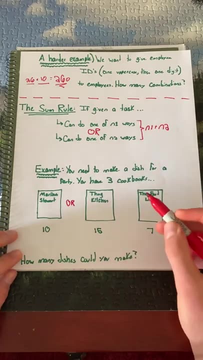 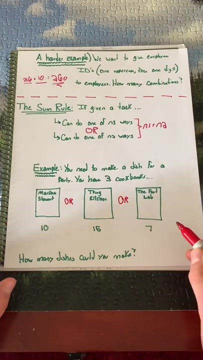 How many dishes could you make? Well, this Martha Stewart cookbook has 10 recipes. or you could use your thug kitchen cookbook, which has 15 recipes, or you could use your food lab cookbook, which has seven recipes. This is the sum rule, and so we know that you have 10 plus 15 plus 7. 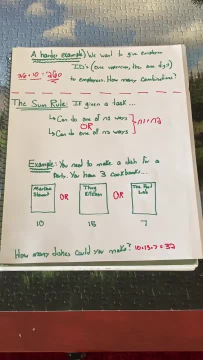 which is 32 dishes that you could make. The product rule and the sum rule are at the base of everything- combinatorics. It's a great idea to make sure you have a firm grasp of them before moving on to some other topics. Thanks so much for watching and good luck.